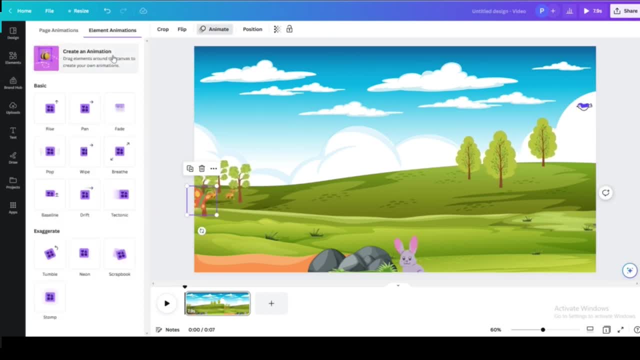 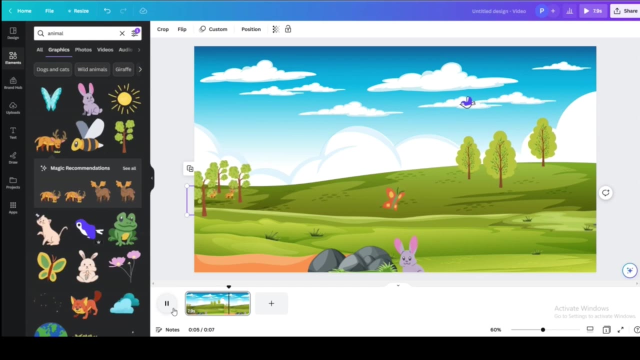 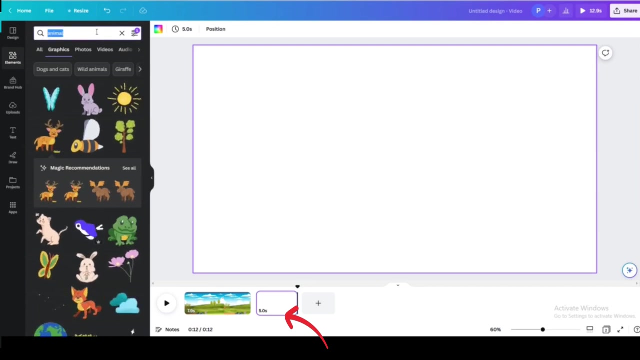 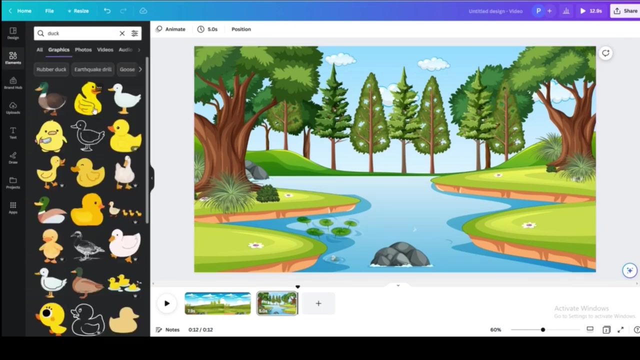 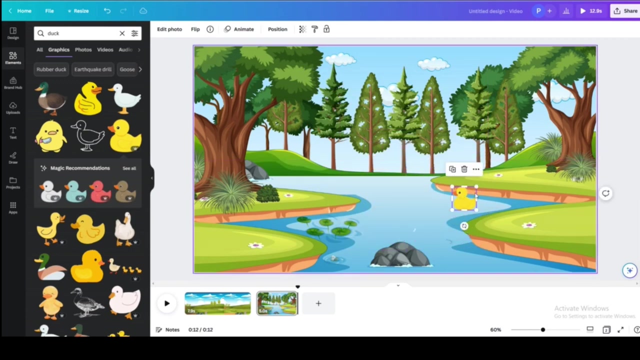 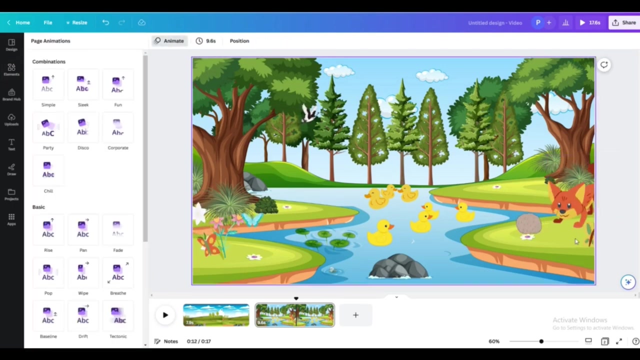 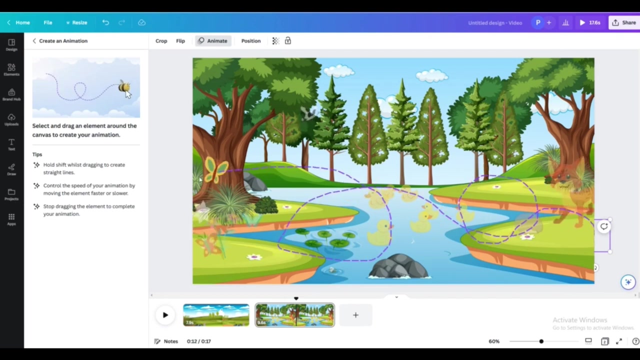 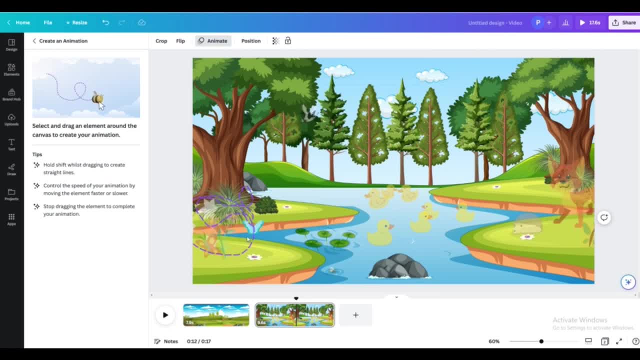 so this is how you animate all the elements you want. okay, all right, we are pretty much done with this scene as well. I hope you are learning how I'm adding the animations to the scene. this is just to give you the like, just a starting point. you can just animate how so ever you want. 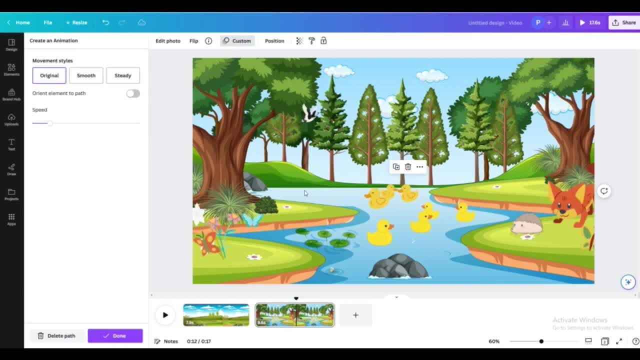 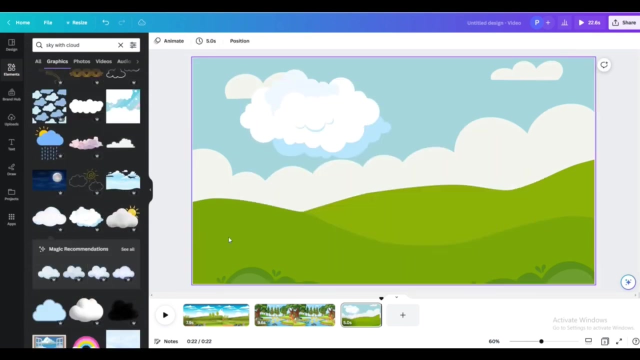 there are hundreds of thousands of ways. I guess you can be creative and make sense more attractive. all right, now we will move to the next scene. this is the master fantasy. if you could see how it actually looks like. okay, all right, now we will add some clouds and this cloud will drift away. 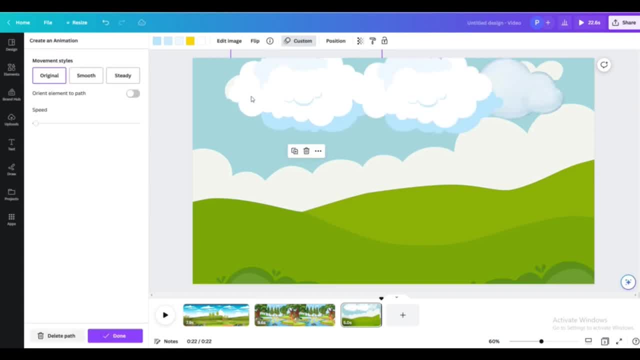 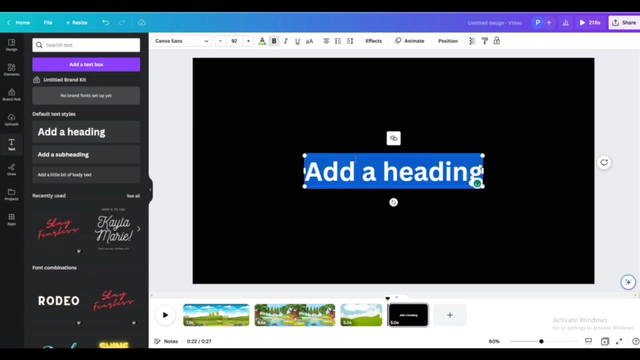 like that. so it is our final scene, pretty much all right, as you can see now, this is how I'm adding animations to the clouds. all right, I'm creating this complete scene here. let's start the finish just to show the people who don't know canva how canva actually works and how you can make it work. but if you're